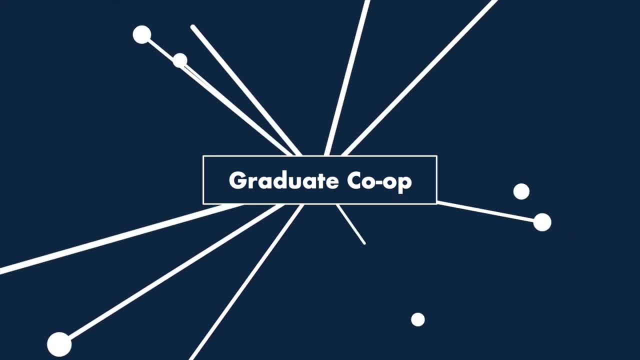 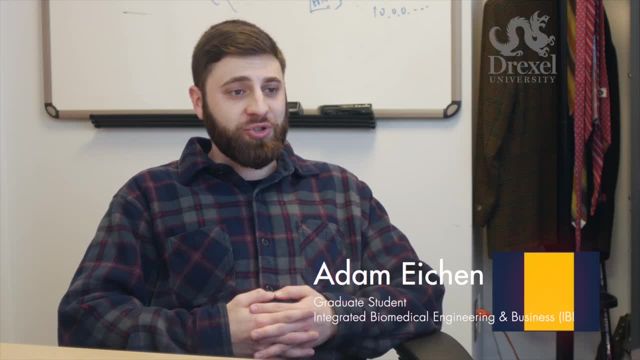 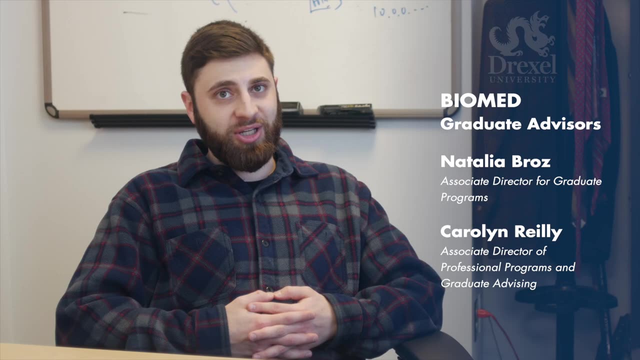 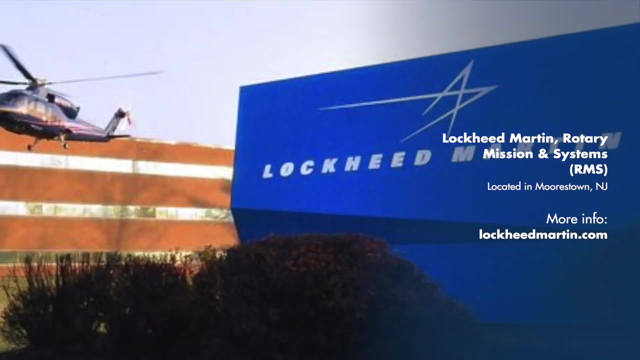 I'm Adam Eichen. I'm pursuing a master's in integrated biomedical engineering and business. My advisors are Natalia Braus and Carolyn Riley for biomedical engineering and Ken Bauer for the co-op. I did my co-op for six months at Lockheed Martin. I worked on artificial intelligence. 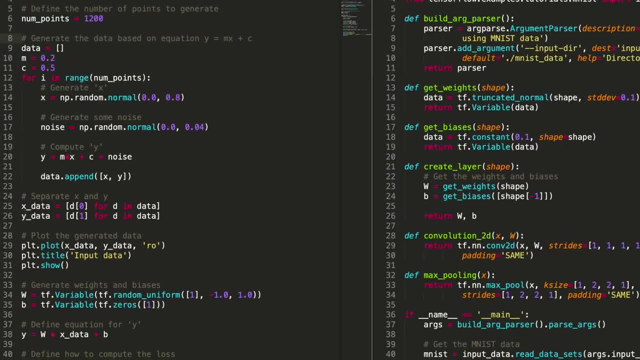 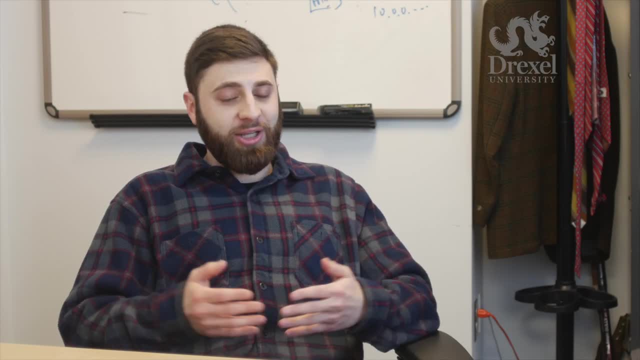 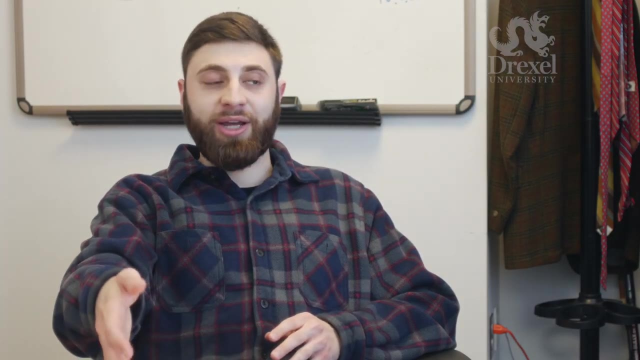 techniques for defense applications. I coded in Python but was given range of pretty much anything. I was impressed with how much autonomy they gave me. I came in on a bit of an exploratory research segment and they said: we want to do this technique. Here's some tools we think can. 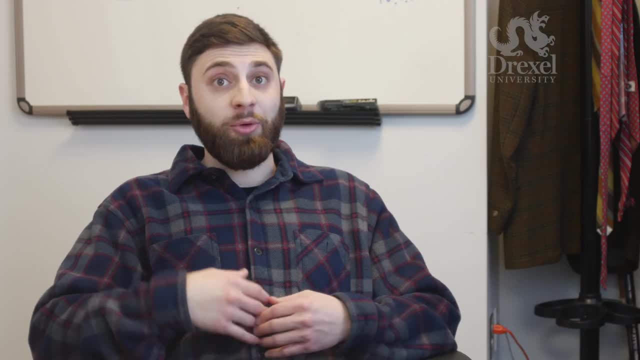 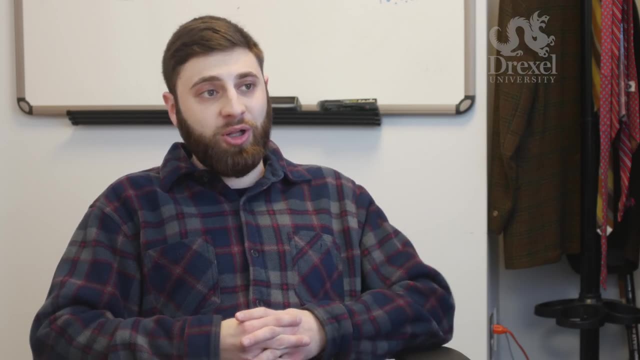 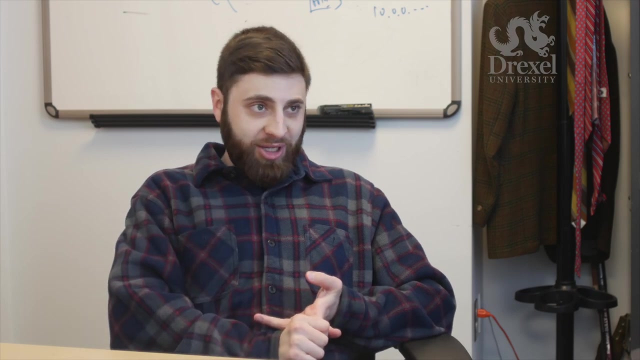 work. Feel free to tailor in whatever you'd like And I would basically show them each week like, oh, I found this. I have this suggestion for your code. They would do the same for me. There was a lot of. It was a really open collaboration. I was not formally trained. I wasn't told no, you can't do. 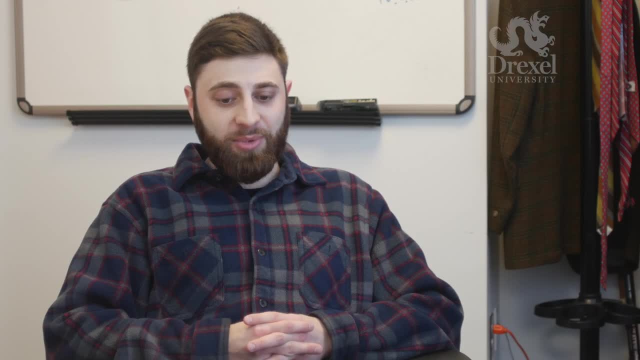 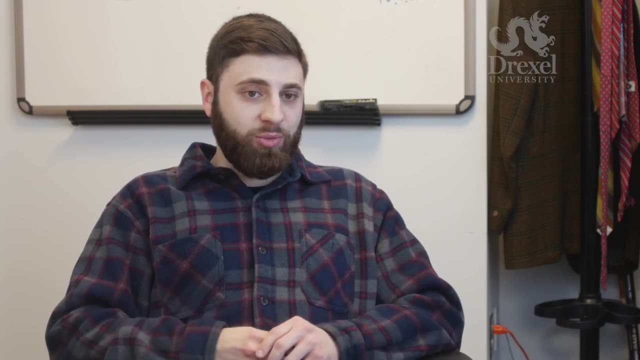 that It was really a nice experience. I had a great time And, besides the fact that they gave me so much room with this project, they really brought me in as if I was already working there. They would bring me to different presentations they have. The company itself does internal. 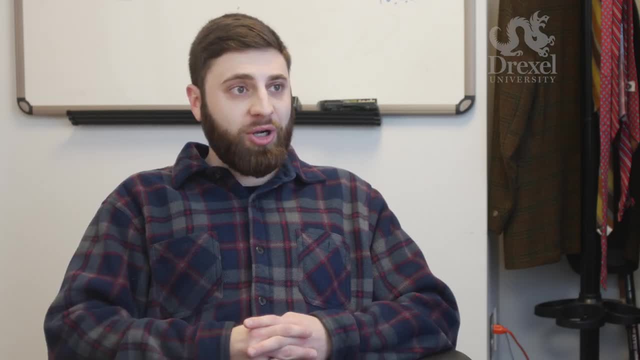 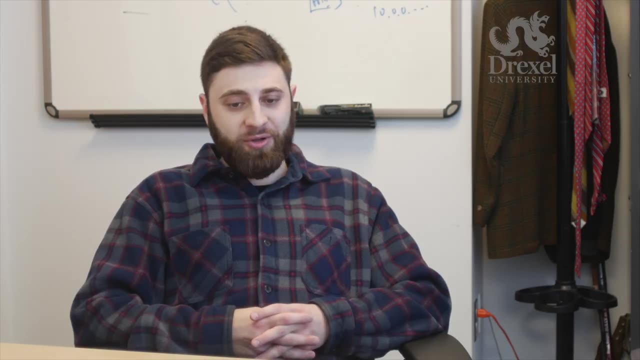 education So I was able to take a couple of their classes. I went to all kinds of meetings with higher ups, lower ups. I got to give my input. They would ask me, which I thought was great, And they were already talking. 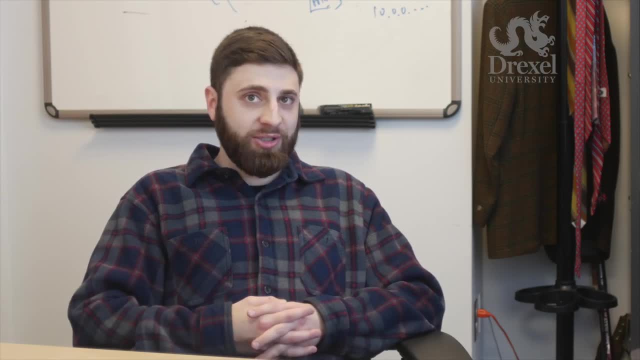 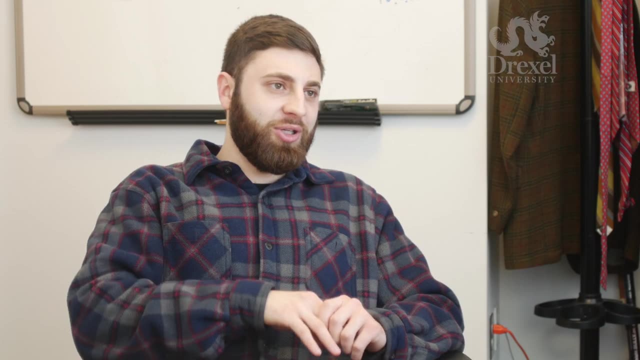 about where I should end up and stuff like that. before the end, Everybody was constantly helping each other with coding aspects. as far as they'd say: oh, if you're looping it like this, you're going to throw it to the CPU like four different times. If you do like multi-pooling, it'd be. 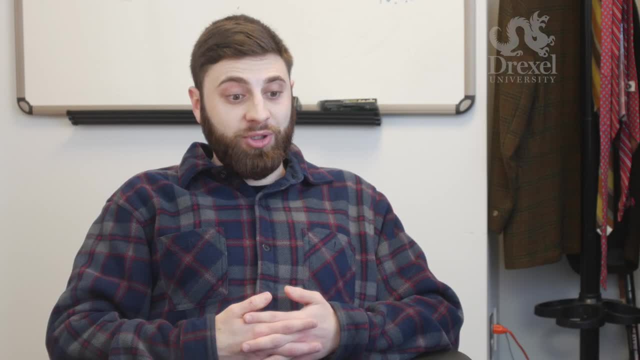 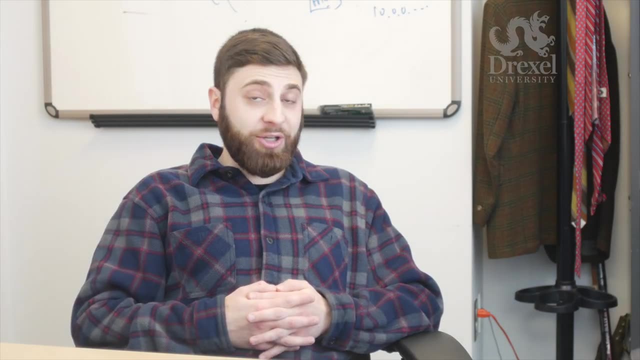 better And I learned a ton. The networking aspect is really where you're going to get the job. A graduate co-op is the absolute best way to essentially preview yourself to a company. I treated it as a tryout. I basically went in there and put everything I had into six. 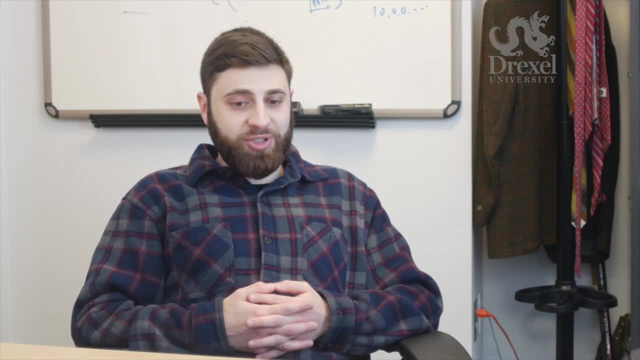 months and showing competence and getting along with the people around you. I actually just got offered.